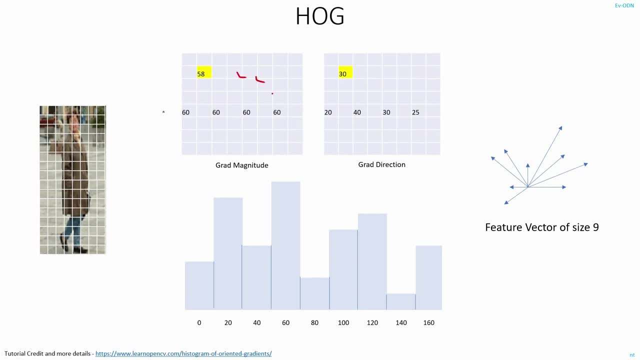 the pixel portions, but I've not shown all of them here. I've shown just few values in this row. Now what we do is we use this gradient magnitude and direction to calculate the feature vectors. Now, if you observe the gradient direction, you will see that all the all the angles, 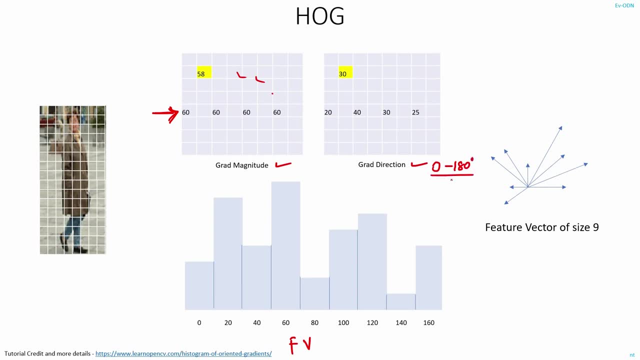 are between zero and 180 degrees. Now these angles I divide into nine different bins. That is from zero to 20 degrees. I'll divide it into one bin, 20 to 40, one bin. 40 to 60, one bin, and so on. The last bin will be from 160 to 180 degrees. Once I do that, I'll check. 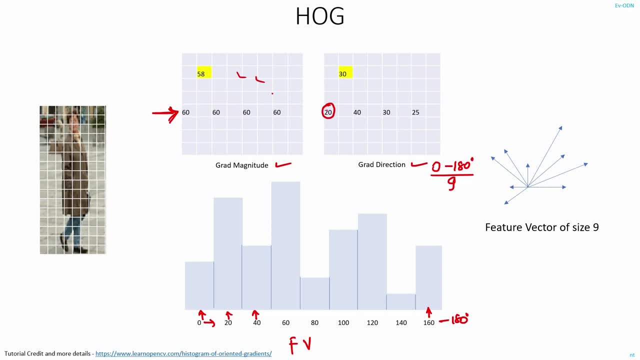 the gradient magnitude, gradient direction at any pixel portion. In this case it's 20 degrees. What is the corresponding gradient magnitude? It is 60. So in the 20 degree bin I'll put a value of 60. Next, here, the gradient direction is 40 and the corresponding gradient magnitude 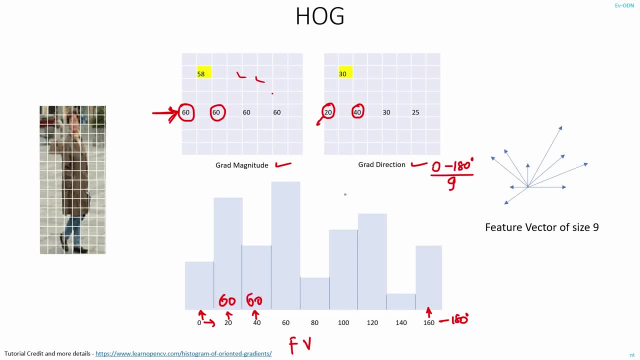 is again 60. So I'll write 60 in the 40 degree bin. In the third example the gradient direction is 30. This is in between right, in between 20 and 40. So what I'll do is, this time I'll 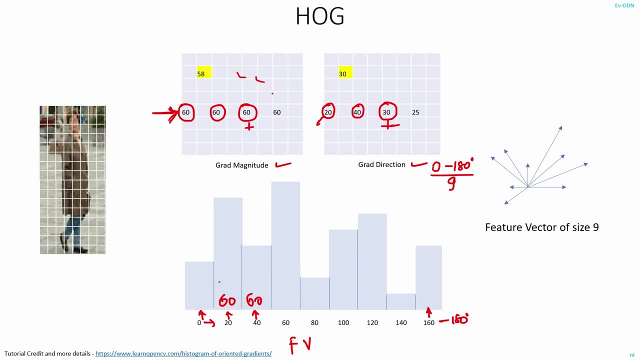 take the gradient magnitude, divide by half and put 30 in the 20 degree bin and 30 in the 40 degree bin. Basically, I'm dividing this value by half and dividing them equally between 20 and 40 degrees bin. Now, what if the gradient direction is 25?? In this case, 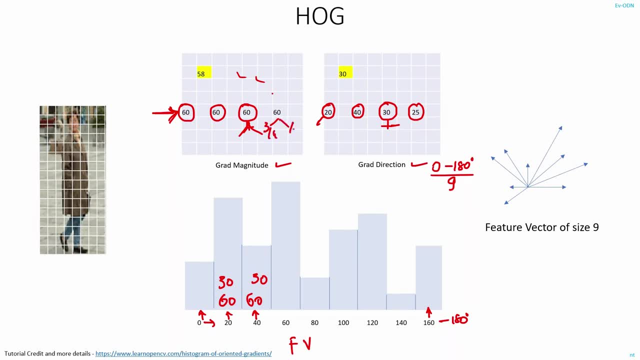 I have to divide it into three, fourth and one fourth. Three, fourth because this 25 degrees is closer to the 20 degree bin than the 40 degree bin, And so now I'll put 45 here and 15 here. The 60, the magnitude 60 is divided into 45 and 15.. 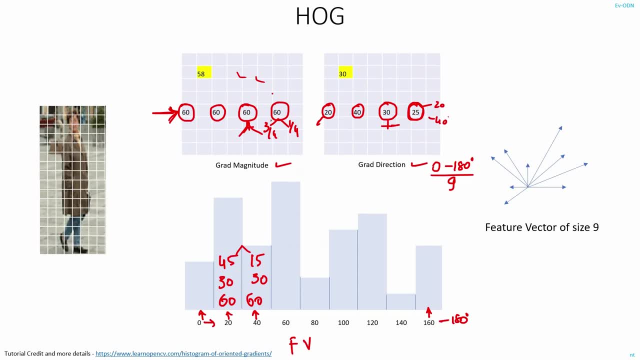 Now what I will do is I'll fill up this bin for all other pixel values, that is, all the gradient, magnitude and directions. Once I do that, I'll sum up the total value in each of these bins. So for 20 degree bin here, the total is 135.. And for 40 degree, it's 105.. 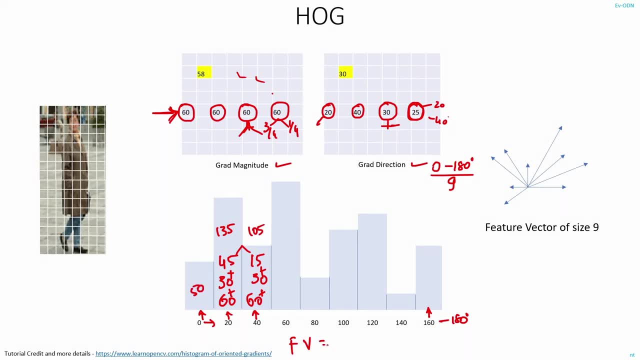 Let's assume for zero degree it's around 50.. Now my feature vector will be just the array of all these numbers, That is, 50,, 135,, 105, and so on. The size will be nine, And when it comes to image processing, we usually express the arrays. 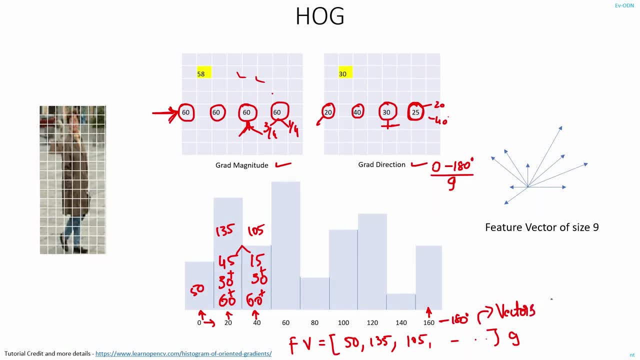 in terms of vectors. So this will be a vector of size nine. It can also be represented as matrix. of size nine is to one that is, nine rows and one column. This histogram can also be represented pictorially in this way. What are these arrows? The first arrow stands for: 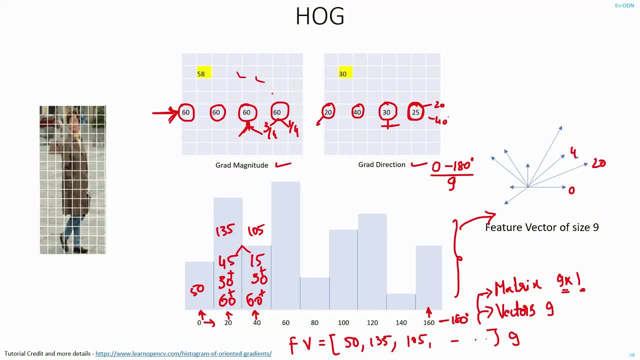 the zero degree bin. This will be the 20 degree bin, 40 degree bin, And the length of this arrow will be proportional to the total magnitude in each of these bins. For example, for zero degree, the length of this arrow will be 50 units, And for 20 degree, 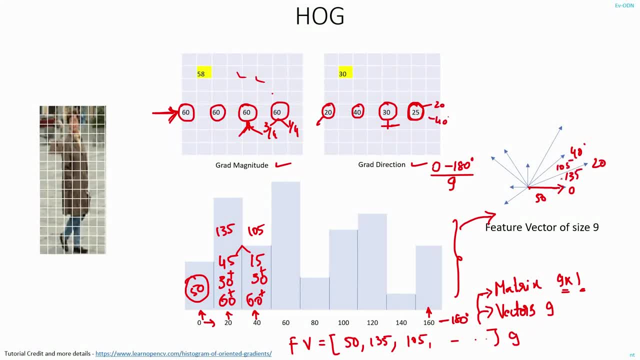 it will be 135,, 40 will be 105, and so on. So here you can see in which direction the gradient magnitude is maximum. In this case it's in this direction it's maximum, But in all other angles, in all other directions, the gradient magnitude change. that is the. 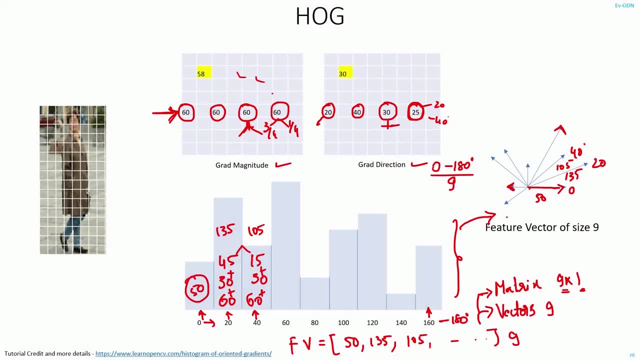 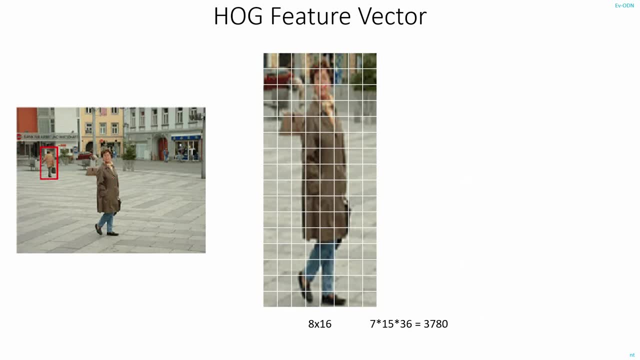 contrast is minimum In other angles. This way I can easily represent the gradient magnitude and direction direction in an image. Now let's just recap what we did. We took an image, cut a small patch of it in the ratio one is to two, that is say, this is 150 pixels and this is 300. Then 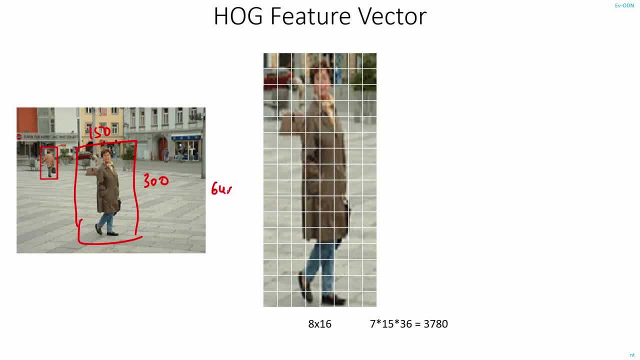 we resize this image, this patch, to 64 by 128.. This patch we divide into eight by 16 grid, And every block of the grid will be eight by eight pixels each. For every block, I calculated a feature vector that is of size nine. Next, what I do is I'll 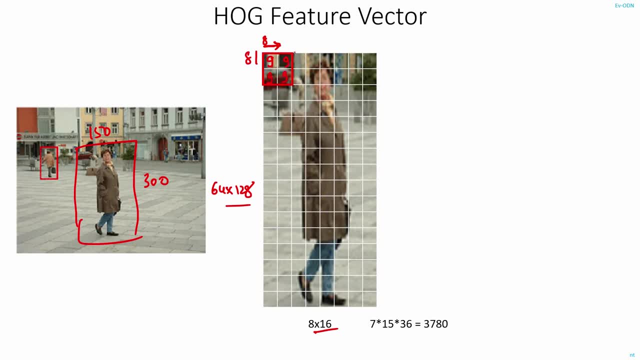 combine four such feature vectors in the adjacent blocks to create a concatenated feature vector of size 36.. Once I do that, I'll move this window one block to the right. Again, I'll concatenate these four feature vectors to give me another feature vector of size 36.. 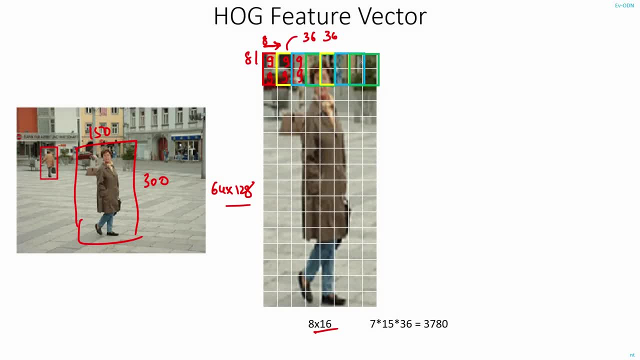 Similarly, I'll do it till the end of the row. In total, how many blocks do I have? I have seven such blocks. Once I finish the first row, then I'll move. I'll move one block down And I'll repeat. 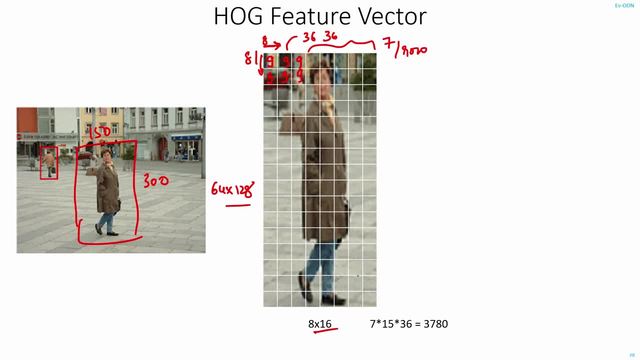 this process. Similarly, I'll do it for all the, all the blocks within the grid. So this will be the my final block, that that I'll be concatenating. So here for a for a eight by 16 grid, I'll end up with seven into 15.. So many feature vectors and each of the feature. 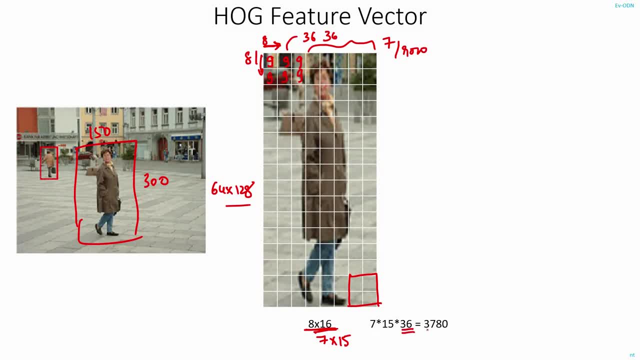 vector is of size 36.. For this patch of the image, my hog feature will be of length 3780.. Now there is. there is one small detail that I left out after concatenating four feature vectors into a size of 36.. I will also normalize it. Now, what is normalization? Let's say you have 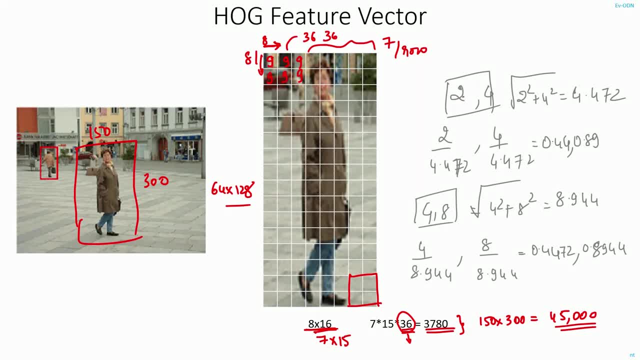 two numbers, two and four, And if and if you want to normalize it, what you do is you'll take the square root of two square and four square, which will give you a number, 4.472.. Then you divide both these numbers by the same number, Then you calculate the square. 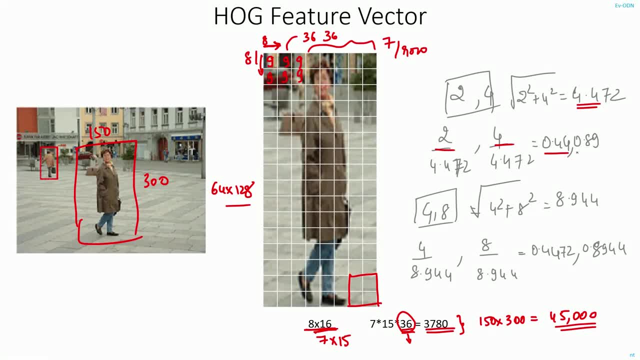 root of two square and four square, which will give you a number: 4.472.. Then you divide both- same number, same value- you will get 0.44 and 0.89. what if you double these two numbers? that is, you will get 4 and 8. again, if you normalize these two numbers, you will get back 0.44 and 0.89. 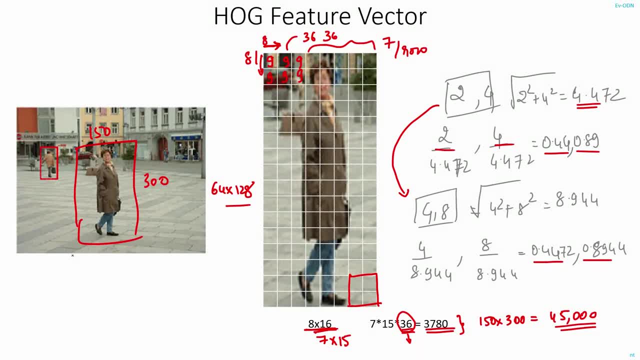 so why is this normalization useful? let's say you take all the pixel values of this image and multiply by 2 to increase the brightness, or say you divided by 2 to reduce the brightness. then if you want to compare these two images, you may not be able to get a perfect match. 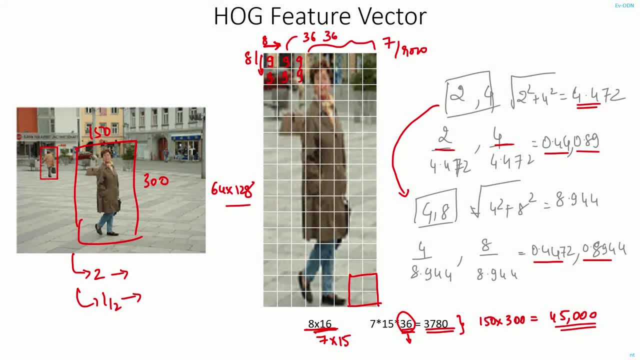 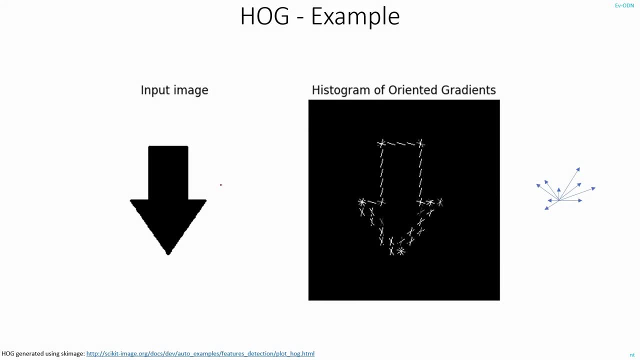 because now the in pixel intensity values have changed. but if you normalize it, your feature vectors will be very similar to each other and it will be easy to compare. now this is one example of hawk feature extraction of an of this arrow image. this i have extracted using the sk image library. 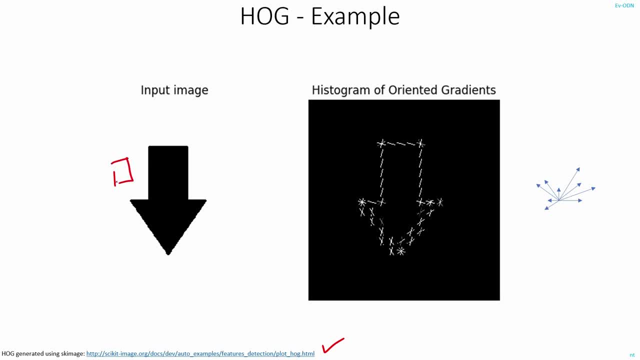 here we can see that in these two patches, wherever the portion is just white or black, there is no change in the contrast in any of these pixels- and hence my hawk feature, that is, my gradient- magnitudes are almost non-existent. and in other places of the image, wherever you are transitioning either from the white 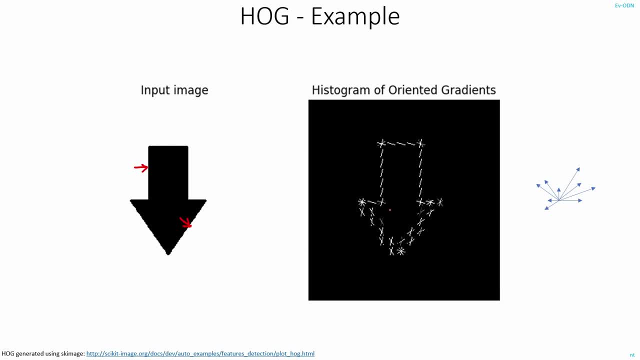 region to the black one, or from the black region to the white one. we can see all the feature vectors being extracted and depicted here and if you are wondering what these marks are, it is nothing but the pictorial representation of the gradient magnitude and direction that we discussed previously and, as we already discussed when you are transitioning from: 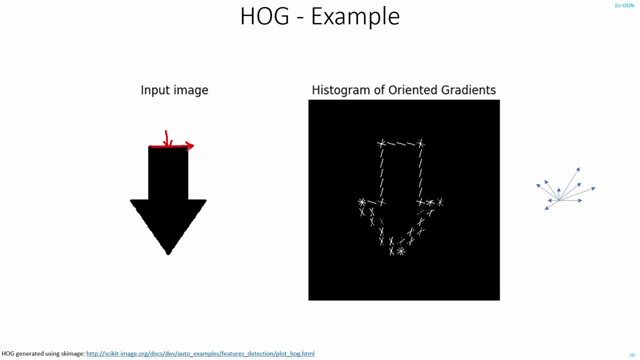 the white region to the black one. here the change in gradient magnitude is along the x-axis mostly, so that's what you can see here, and in this edge the change is in the y-axis, so even here you can observe the same thing. one more observation is that this corner looks very different from this one. 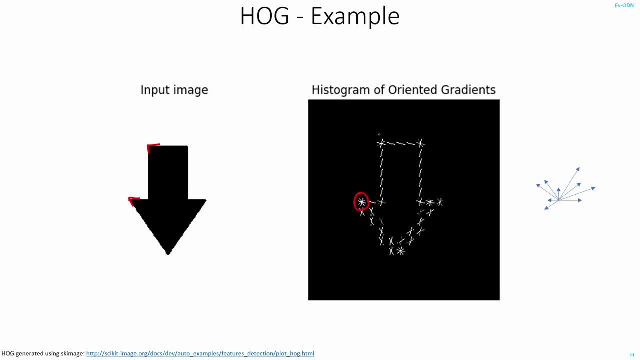 so even this change, the difference in how the corner looks, can be observed using these feature vectors. and the last observation is: even if you take the edges that are inclined, that is, this is a backward inclination and this is a forward inclination- the gradient magnitude or the feature vectors are not the same. so even if you take these features, they 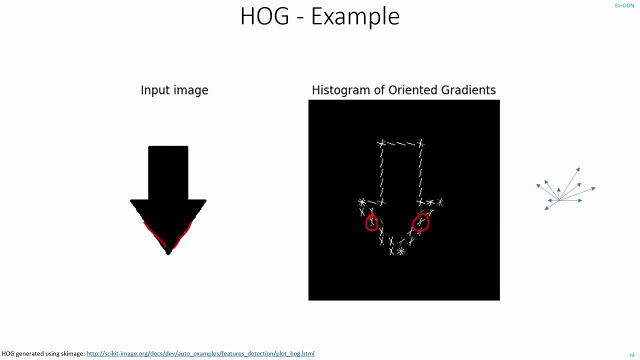 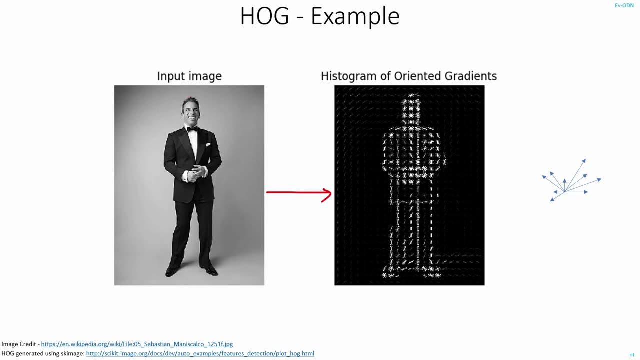 vector representations look similar, but they are in a different direction, So you can even know, based on this, in which way the edges are aligned. Another example of hawk features being extracted on a human, human body: Here we can clearly see that wherever there is a face or hands or any other interesting portions of the image, 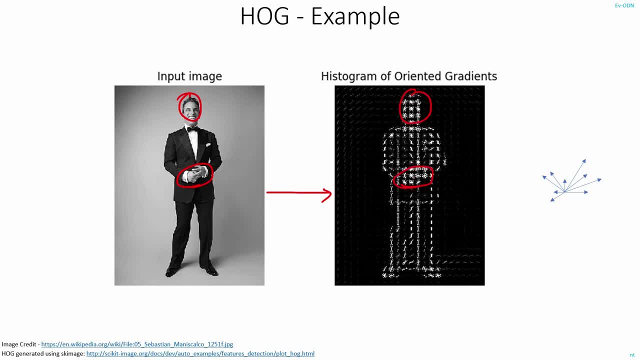 the hawk features are clearly able to extract them and all the other patches of the image where there is not much information, we can see that even the gradient magnitude values are very less, And in places where there is a uniform pixel intensities, there is not much change here. 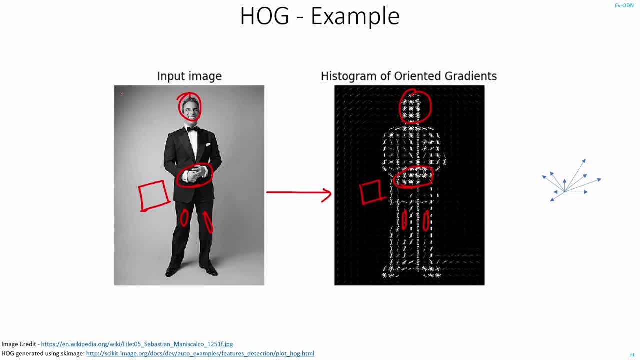 Even the hawk features depict the same thing. The last thing that we discussed was that it's not necessary that the change in magnitude should be very sudden, like in these edges, But it can also be gradual, as we can see in this portion, So the same thing can be seen. 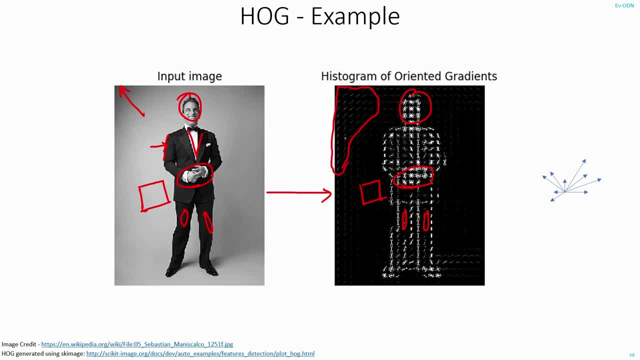 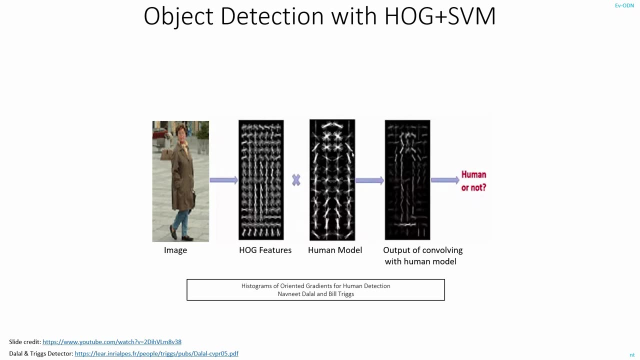 here are extracted, but the gradient magnitude values are small compared to other portions in the image. this, in short, is how hawk feature extraction works. now you might ask: how will i? how will i use it in my practical situation? now, let's say you want to do some object detection. let's take the task of detecting humans from images. how will you do it? 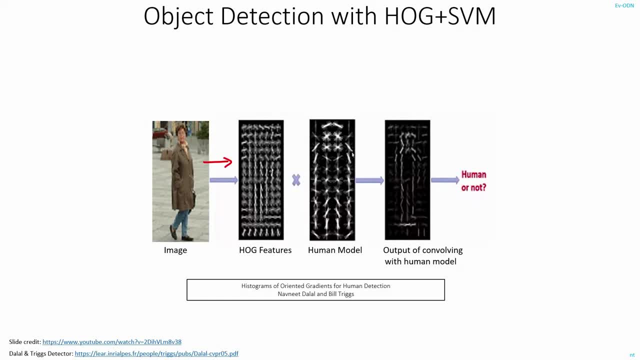 what you have to do is, given any patch of the image, you extract the hawk features. once you extract, you convolve these features with the human template, that is, this is a filter for how the hawk features for human should look, and once you do the convolution, you will get an output.